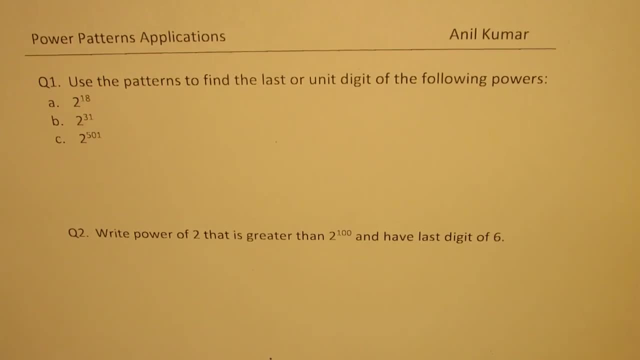 I'm Anil Kumar. In this video we are going to explore the power patterns. Now, these are very important and useful patterns and many times in competitive exams and tests we see a question related to these patterns. To begin with, we'll look into the patterns with powers of two. Question number one is: use the. 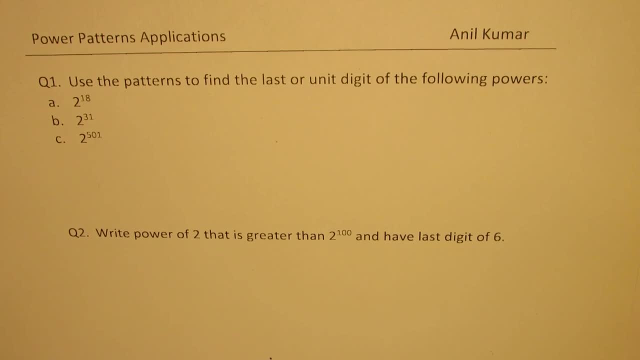 patterns to find the last or unit digit of the following powers. And question number two is write power of 2 that is greater than 2 to the power of 100 and have last digit of 6.. So unit or the last digit is the units place digit right. 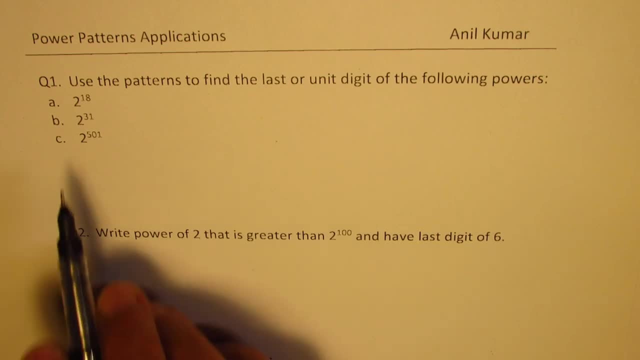 Okay, so to get the pattern, let us write down few powers of 2 and see what they are and what kind of pattern do they have. So if I write 2 to the power of 1, we know this is equal to 2, right? 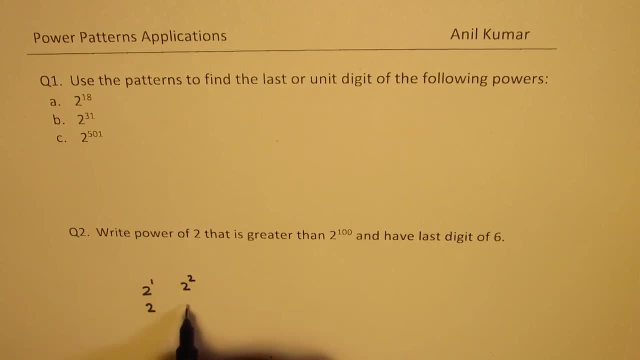 If I write 2 to the power of 2, we get 4.. 2 to the power of 3 is 8.. 2 to the power of 4 is 16.. And when I get 2 to the power of 5, you will see it is 32.. So I'll write. 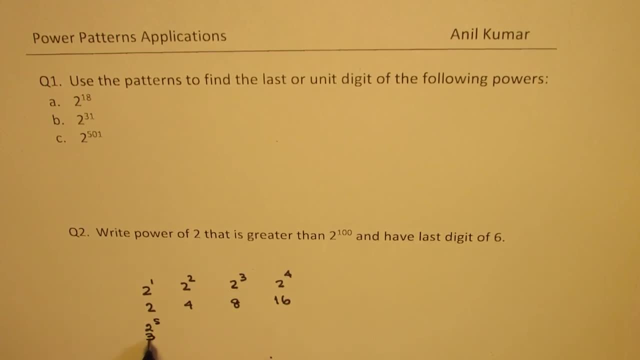 2 to the power of 5 here. So 2 to the power of 5 is 32.. 2 to the power of 6 is 2 times 32, 64.. 2 to the power of 7 is 2 times 64.. So it is. 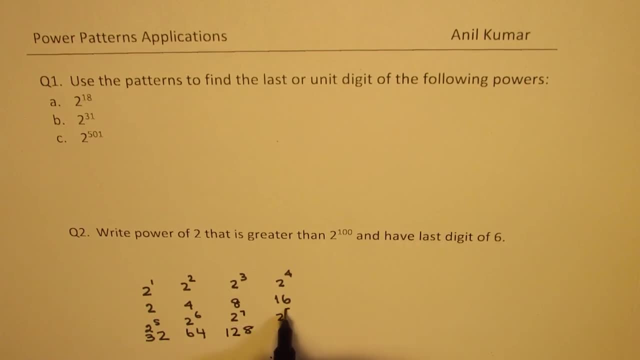 8 and 1, 128.. 2 to the power of 8 is 2 times 128., And so we get 256.. So if you look into the last digit, so last digit, 2 and 2 matches right, Then we have. 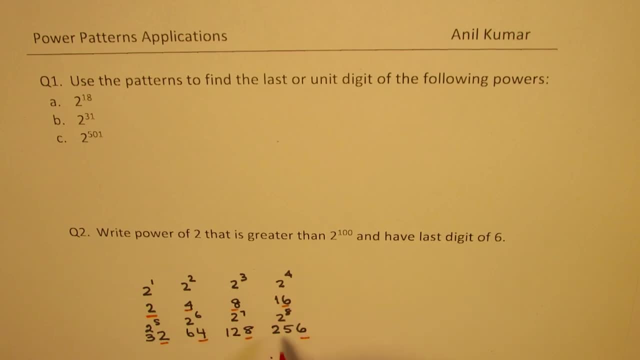 4 and 4.. and eight, six and six. now this is what we call as the last or the unit digit. so in any power of two we find a pattern right. this number two, four, eight, six repeats. so if the power is a multiple of four, in that case the last digit is six. 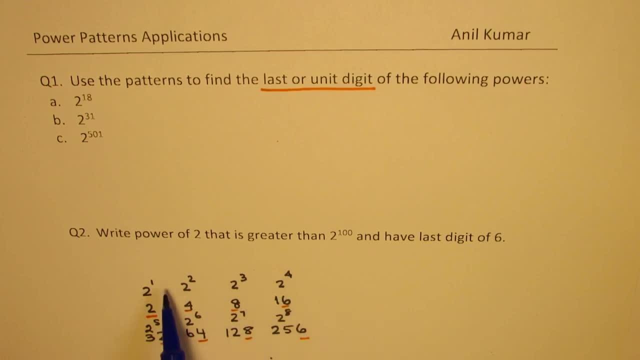 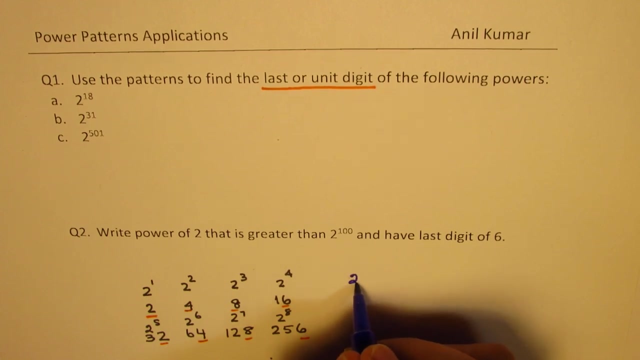 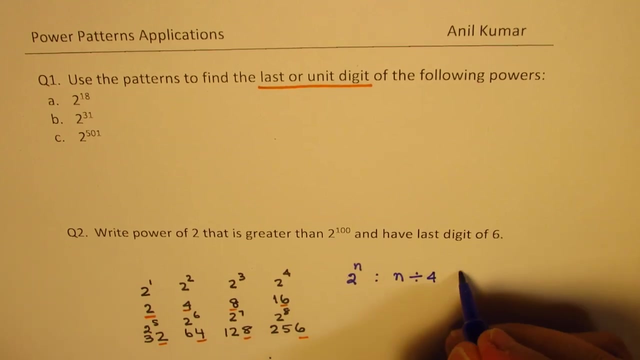 right, but in case there is a remainder, then if the remainder is one, then the last digit is two. do you see that? so basically it is based on remainder. so whenever you have two to the power of n, then what we do here is that we'll divide n by four and then check remainder. 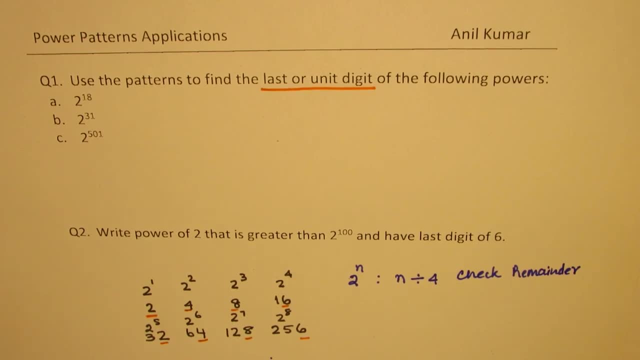 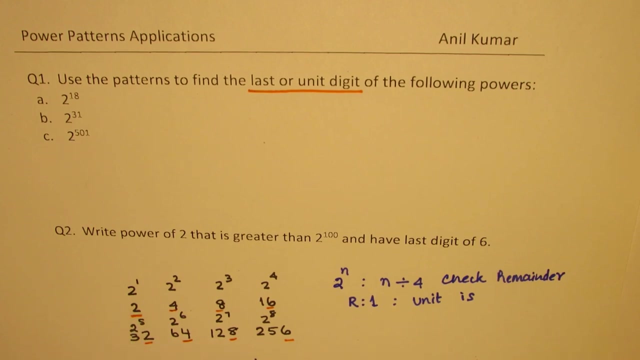 correct now if the remainder is one, if the remainder is, let me say, remainder is one, in that case the unit place is unit is the unit place is two. do you see that for a one remainder unit places two, as in two or in thirty two. so the 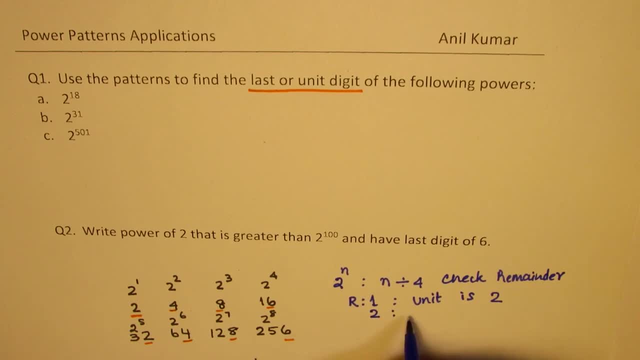 unit is two, but if the remainder is two, then the unit is one, then the limit is four, and in that case a three place is two, and также the unit is one, and so this is the unit one, Metal1 in at the times. 若 is the unit. 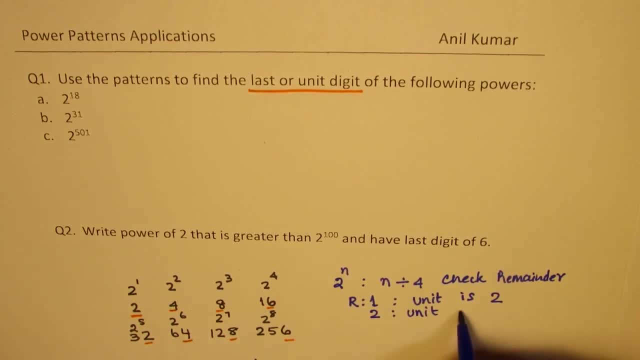 eight, nine, then okay, 若 is number twelve, then out comes the e, then in drunk the back comes the one in 若作. no see that we repeated Correct y, then a. so will not. otherwise 若 is divided. 若 did not bite 若. the remaining, I should say unit place value is 4. if the remainder is 3, in that case unit is 8. if the 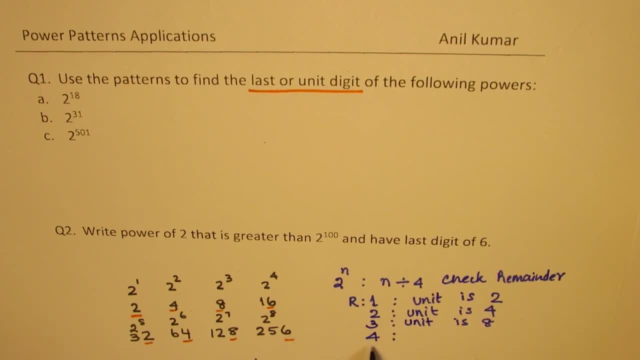 remainder is 4. now can the remainder be 4? you are dividing by 4, so remainder cannot be 4, right? so 4 divided by itself will be 0, so i should write this as 0. so if the remainder is 0, that is, if it. 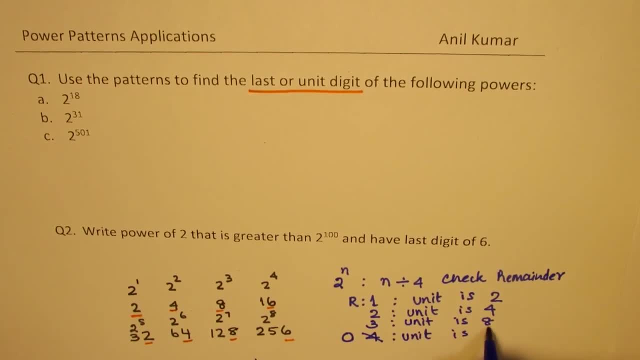 is a multiple of 4, then the unit is 6. so that is the pattern which is being followed. perfect. so we have to use this pattern rule to answer our question. so now let us see how to answer it. it says: use the patterns to find the last or the unit digit of the following powers. now the power. 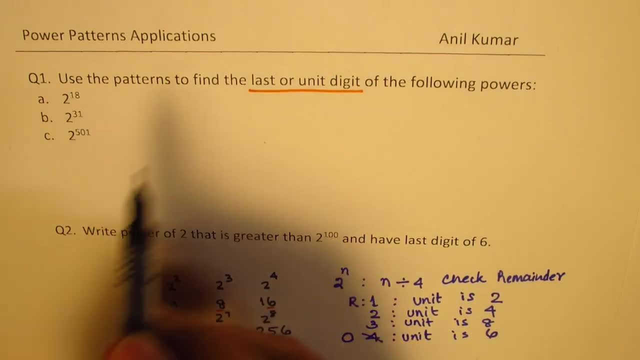 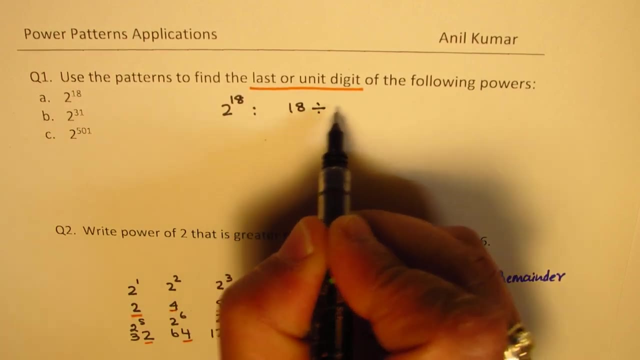 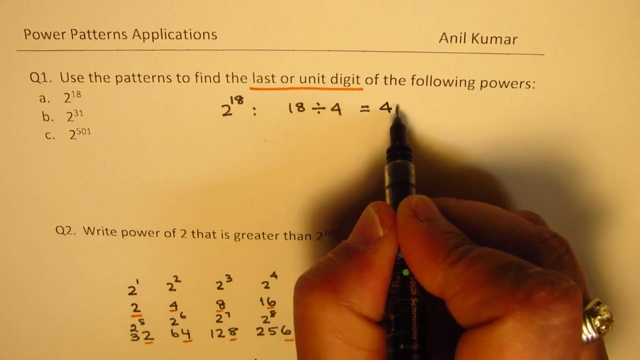 here is 2 to the of 18. so what we are going to do, so to test 2 to the power of 18, what you have to do is you have to divide eighteen by four and check the remainder. so so four goes four times. so it is four, remainder two now, since the remainder is two. so what is the last? 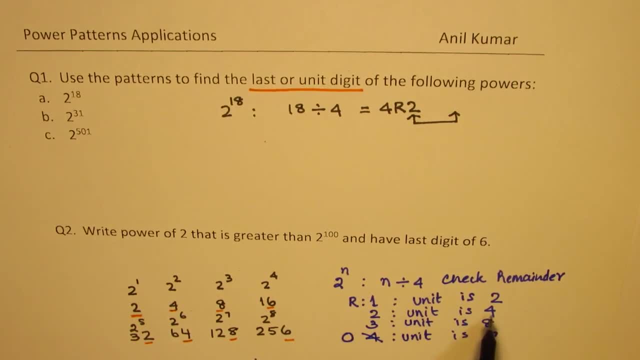 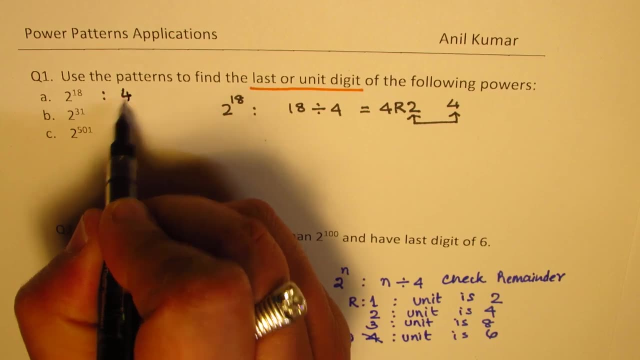 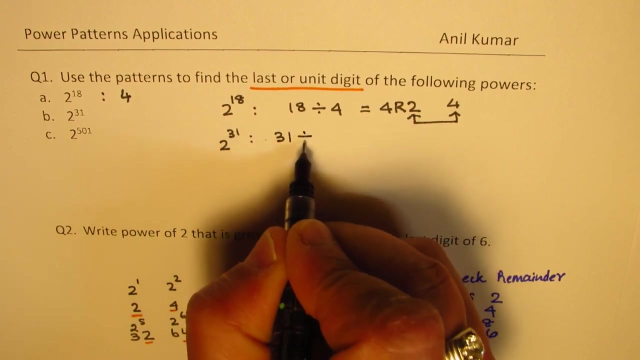 digit for two. the remainder, the last unit, should be four, right, so we have four as our answer. so So the last digit in this case is 4.. Is that clear? Now, in case of 2 to the power of 31,, you have to divide 31 by 4.. 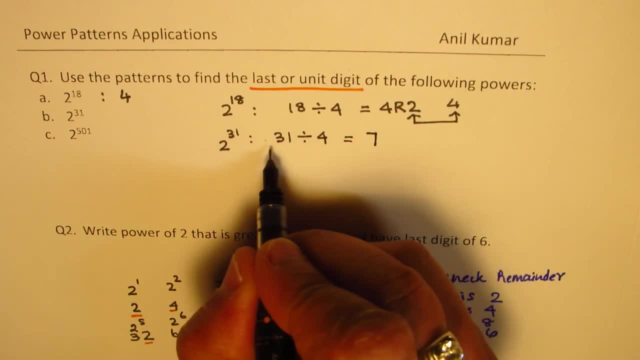 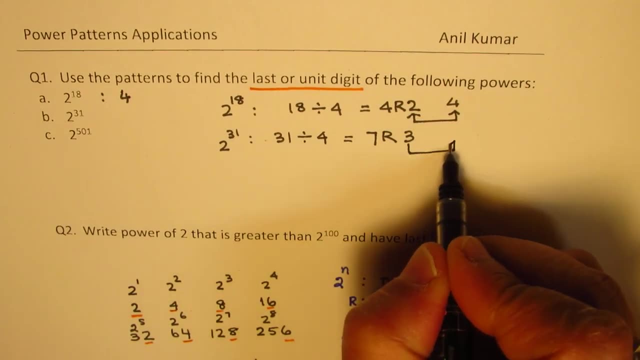 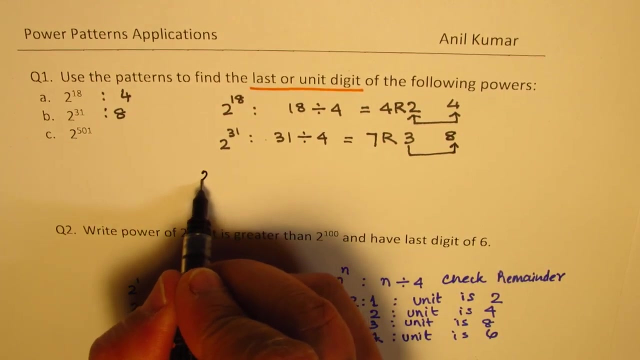 So when you divide 4 times, 7 is 28 and the remainder is 3.. For 3, the last digit is 8, and so we get the unit place as 8.. And so this answer is 8.. And for 5 or 1,? so when you do 2 to the power of 5 or 1,, then divide 5 or 1 by 4.. 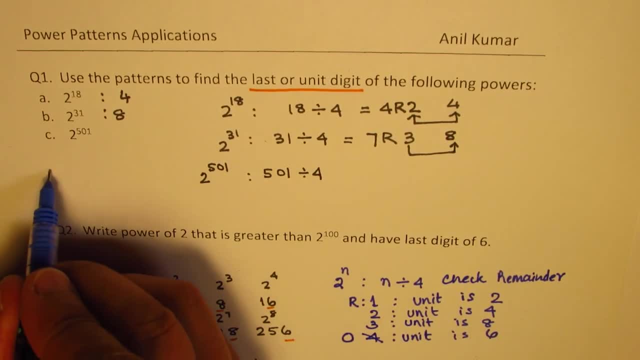 So if it is a difficult division you can do it on the side. So I have left this space for the same. So we are dividing 5 or 1 by 4. So 4 times 1 is 4. We get 10 here. 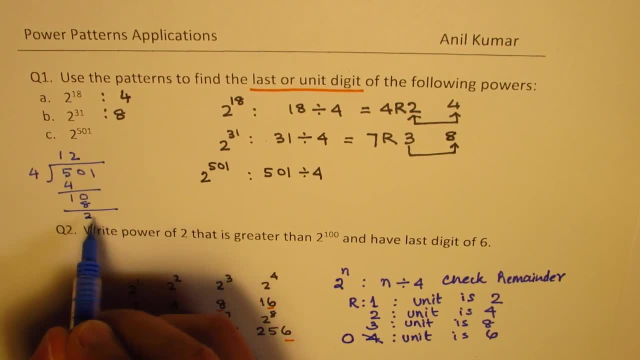 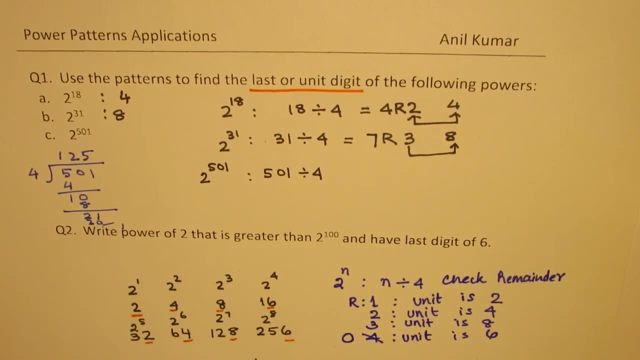 4 times 2 is 8. And we get 2.. Bring down 1.. 4 times 5 is 20.. And so the remainder is 1.. So we can write this as equal to 125, the remainder 1.. 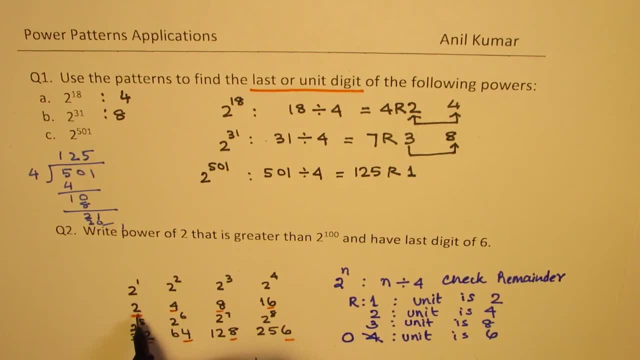 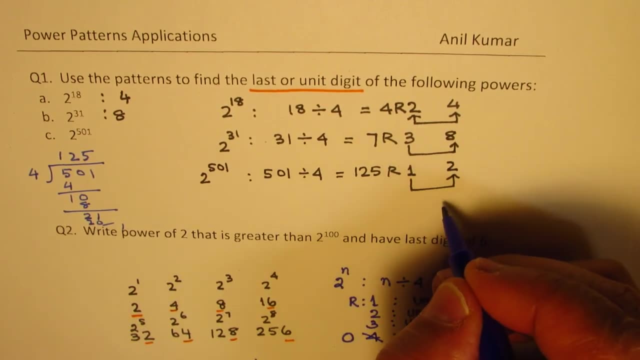 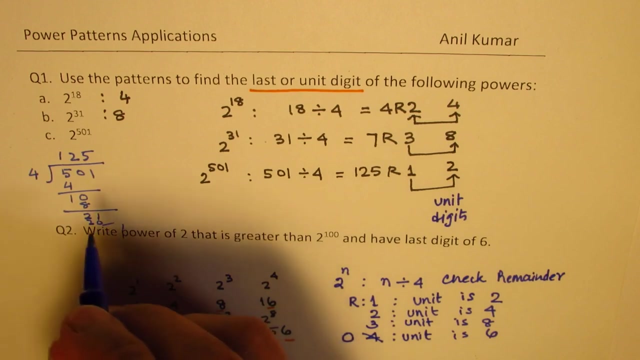 Since the remainder is 1, the 1's place should be 2.. So we get this answer as 2.. So these are 1's or unit digits, The last digits which we have shown above, And so we get the answer 24.. 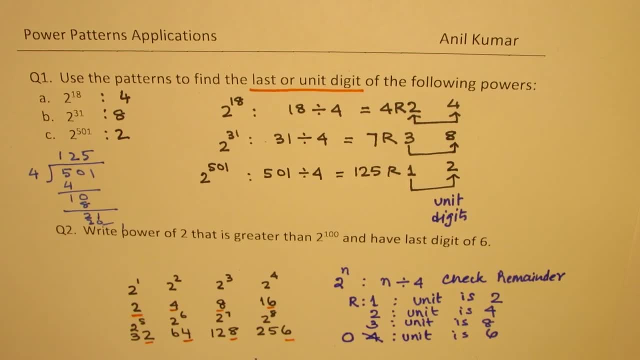 Now let's look into question number 2,, which is right, power of 2,, that is, greater than 2 to the power of 100, and have last digit of 6.. Now, last digit of 6 means multiple of 4.. 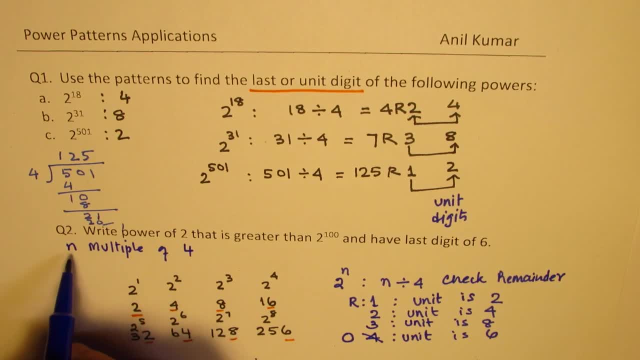 What? the index or the exponent n is multiple of 4, correct. Now 100 is a multiple of 4.. So the next higher will be 104, right. So we could write this as 2 to the power of 104.. 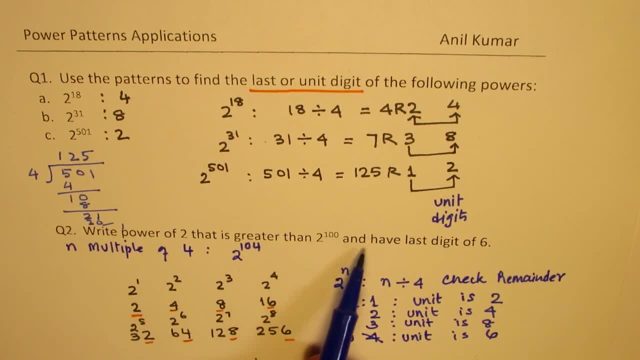 So write the power of 2 that is greater than this and have a last digit of 6.. So 2 to the power of 104 will have a value with last or the unit's digit as 6, right, Since it evenly goes in 4..